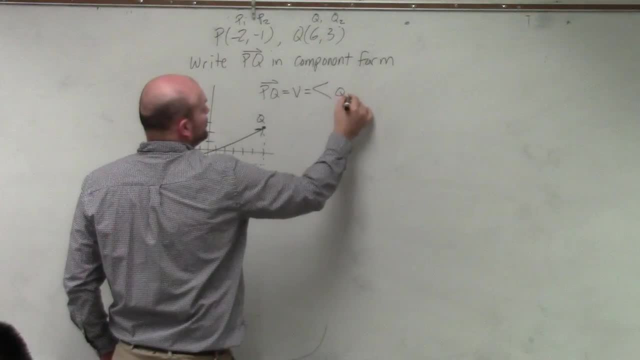 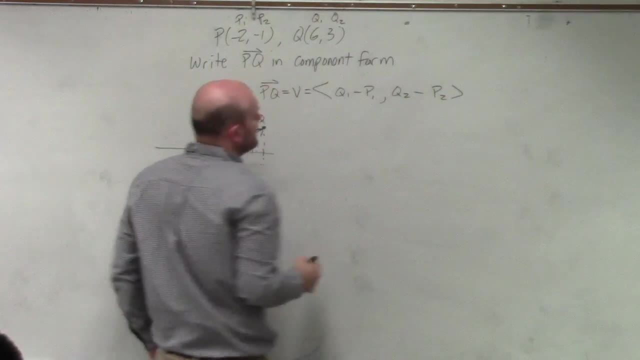 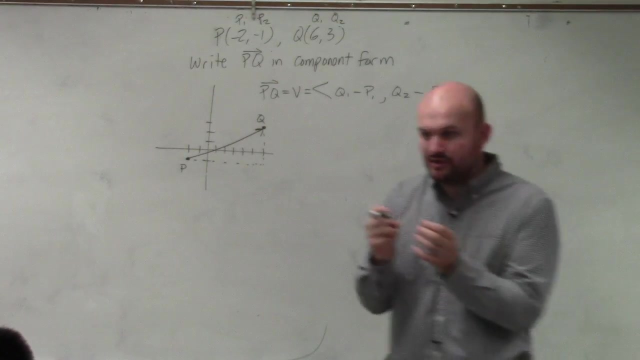 with the change in my Y coordinates. So I'm going to do Q1 minus P1, comma Q2 minus P2.. Again, all I'm simply doing is finding the change. all I'm doing is finding the change in the X and the Y coordinates. okay, 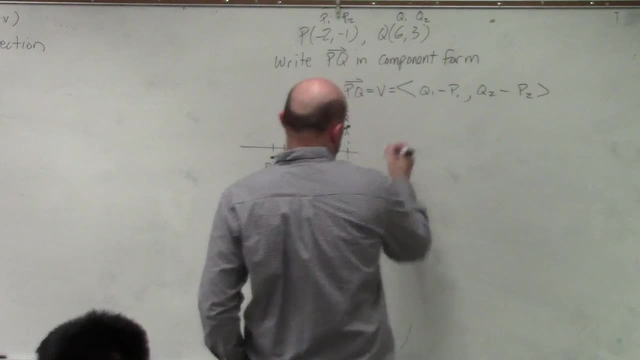 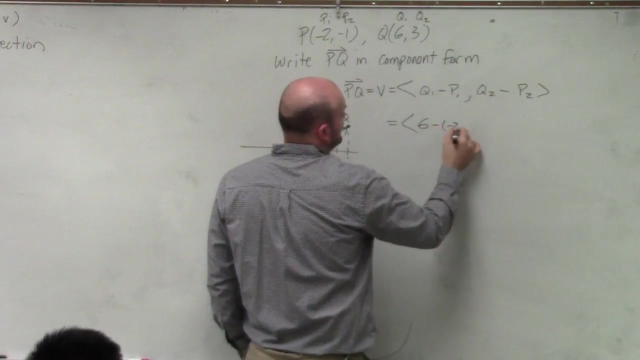 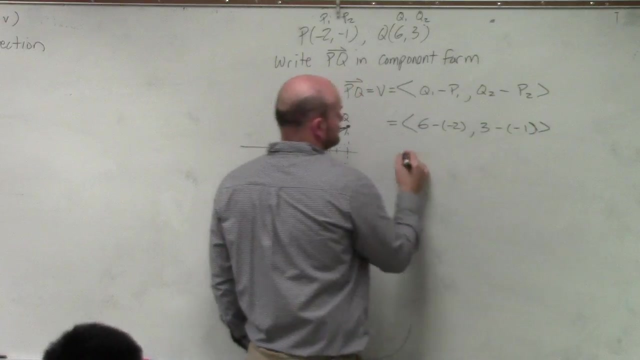 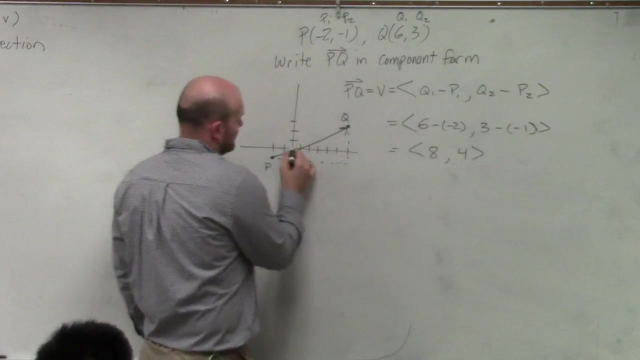 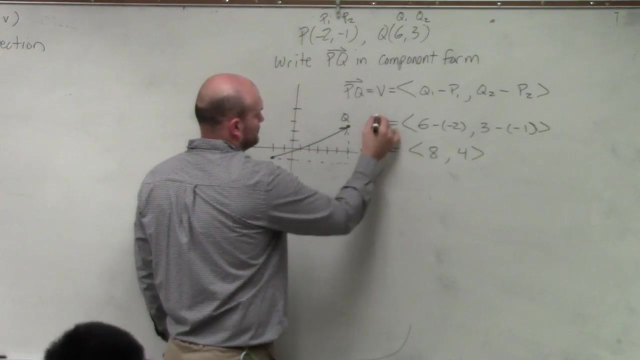 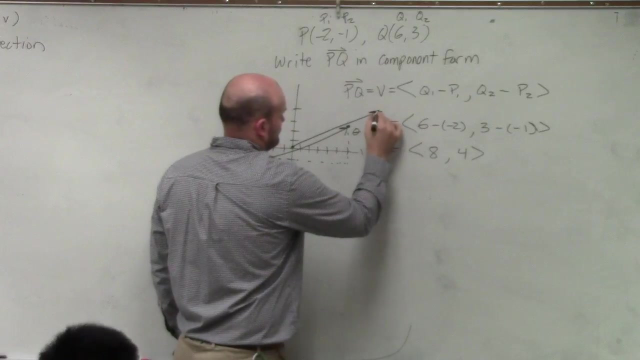 So, and I'm going to call this vector, instead of calling it vector PQ, I'm just going to call it v. So therefore, I have 6 minus a negative, 2, 3 minus a negative 1.. So 1,, 2, 3, 4, 5, 6, 7, 8.. 1,, 2,, 3, 4.. Now, I know my graph is not perfect, but do 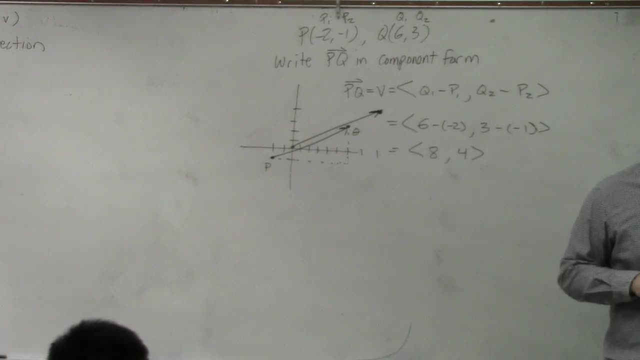 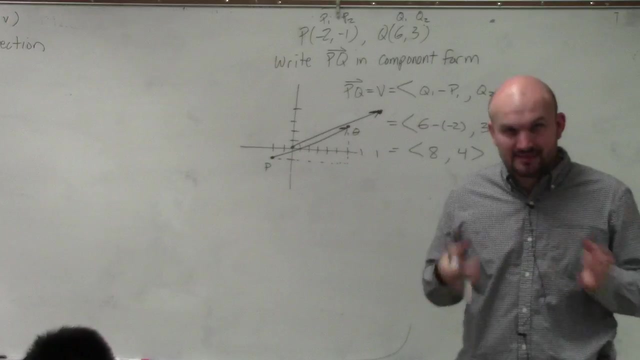 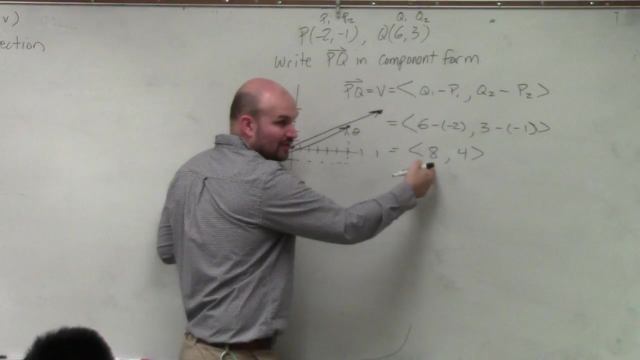 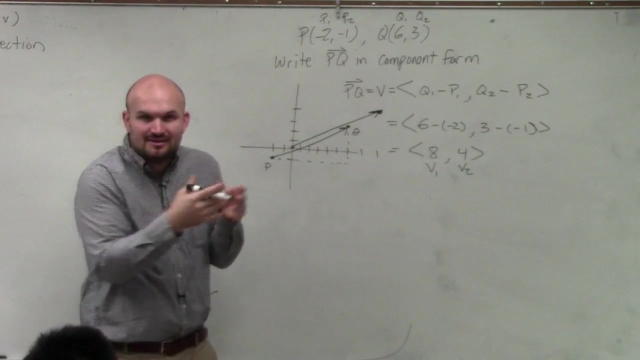 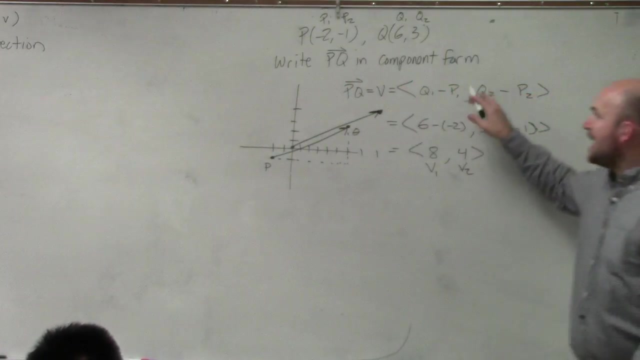 you guys kind of see that the vectors look pretty much the same, right, They have about the same magnitude and they have about the same direction, correct? The difference is that my vector in component form, which I could say that's v1 and that's v2, those are my two components- has an initial position at where Zero. right Now it's really helpful and again I'll explain that. The other thing I want you guys to notice is I 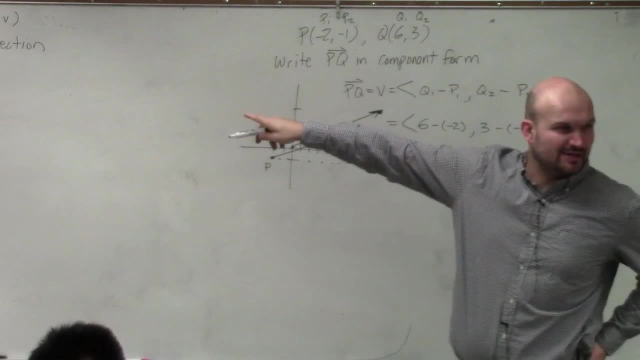 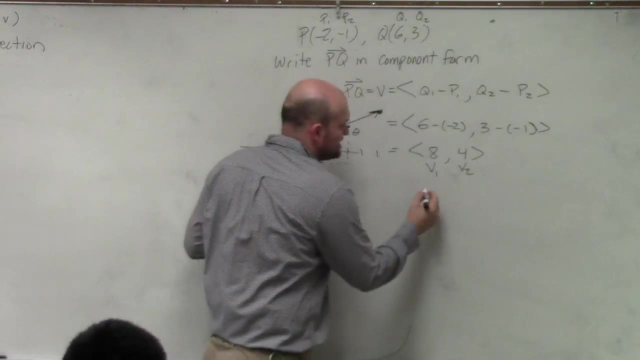 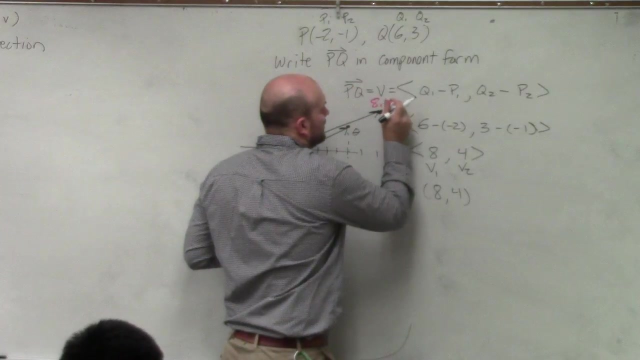 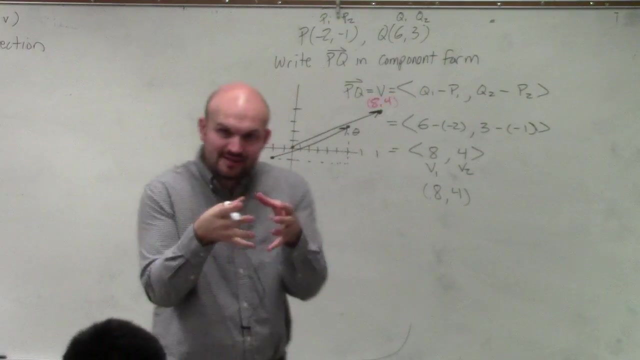 represented my vector. you guys can see in component form. Look what I used. I used component form as kind of these slanted parentheses. right Now let's look at slanted parentheses. kind of reminds me of regular parentheses, But regular parentheses gives me a point- 8, 4, which is right there. So the difference between a parentheses 8, 4, gives you a coordinate point. Slanted parentheses- 8, 4, gives you a coordinate point. 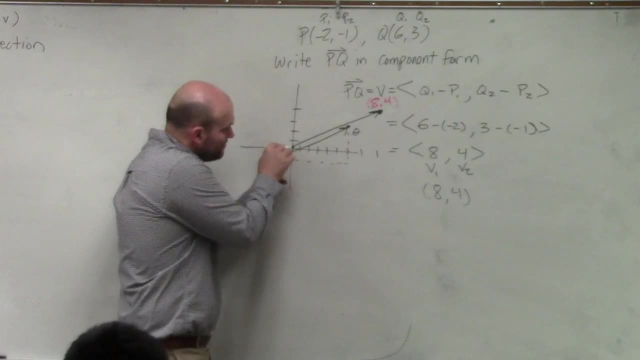 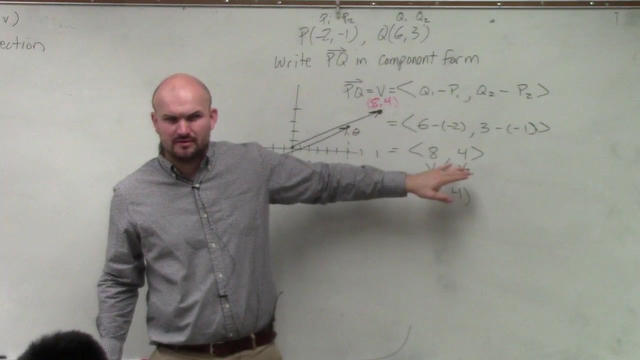 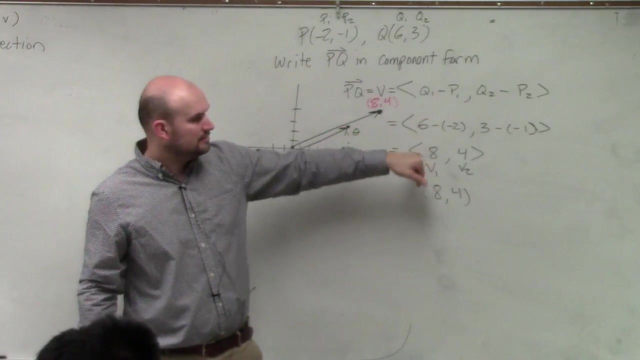 8, 4 gives you a directed line segment from 0 to 8, 4, which is what we call our vector. Does that make sense? A little bit, kind of, Okay. So just remember, this is saying that's a directed line segment from 0 to the point 8, 4.. Directed line segment, That is just a point Okay. So now we found component form.